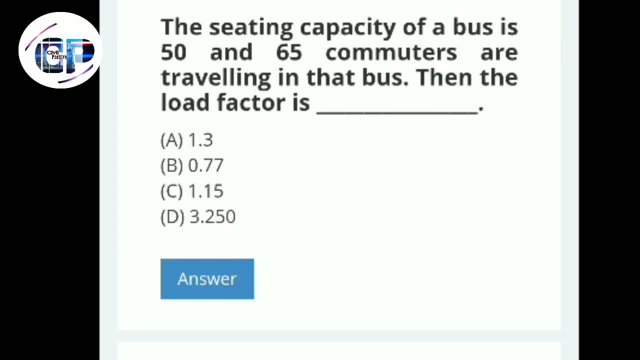 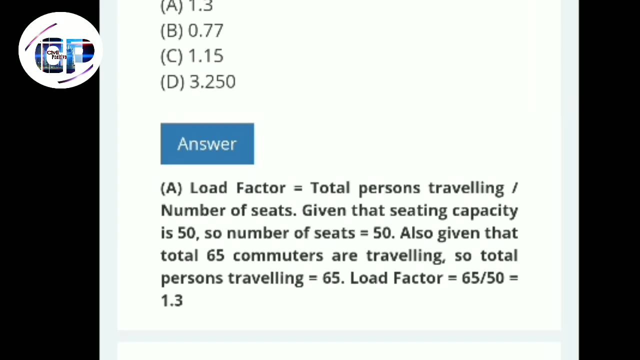 50 and 65 commuters are travelling in that bus, Then the load factor is D 1.3,, 0.77,, 1.15 or D 3.250.. Answer: A 1.3 Load factor equals to the total person travelling divided by number of seats. 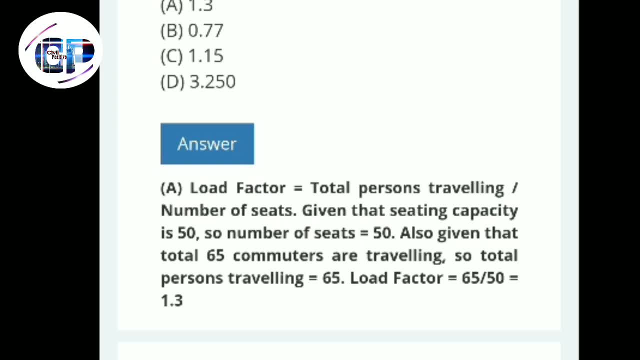 Given the seating capacity is 50,, so the number of seats is 50.. Also, given that the total 65 commuters are travelling, so the total person travelling is 65.. To calculate the load factor of 65,, if we divide it by 50, then it is 1.3. 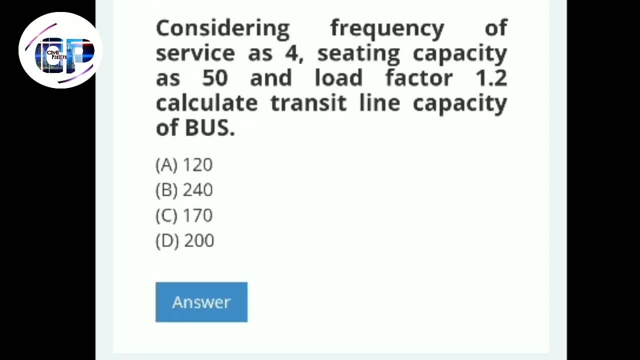 Answer A is right: 1.3.. Considering frequency of service is 4, seating capacity is 50, load factor is 1.2,, calculate the transit line capacity of bus. Calculate the transit line capacity of bus, That is what is the total transit line capacity of bus. 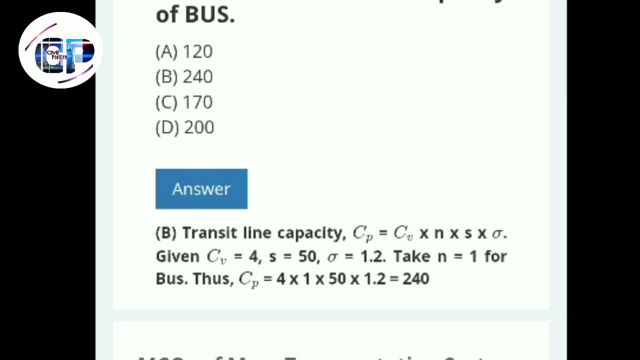 Now the answer is B 2.40.. So transit line capacity equals to CB, into N, into S, into sigma Given CB is given to you, which is 4, which is given as service, S 50 is given the seating capacity is 50, so sigma 1.2 is given to you. load factor: 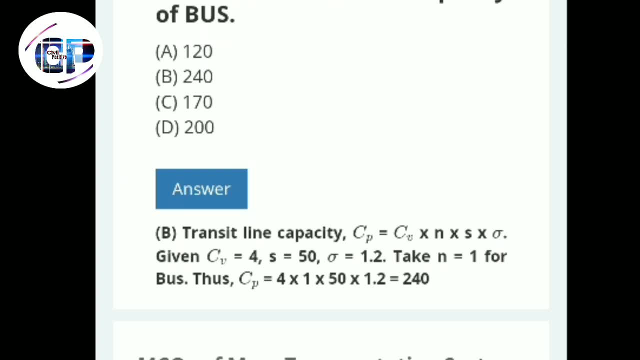 Taken, N equals to 1 for one trip, Fourth bus. Thus to calculate, CB equals to 4 into 1, into 50, into 1.2.. So you will get 2.40.. The answer is B is right. 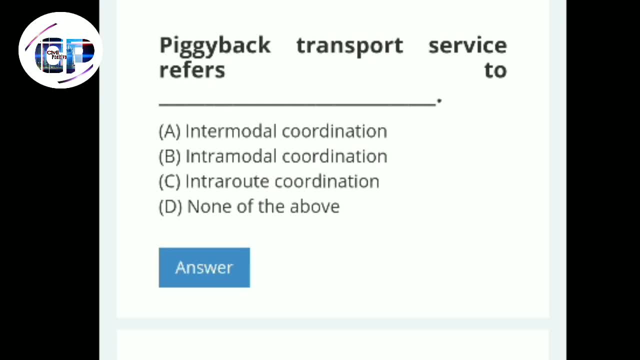 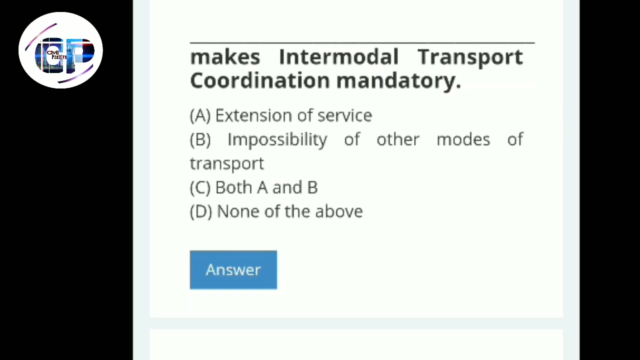 Piggyback transport service referred to intermodal coordination, intramodal coordination, intraroute coordination. none of the above Answer A intermodal coordination. Thus make the intermodal transport coordination mandatory. Extensive of service Impossibility. 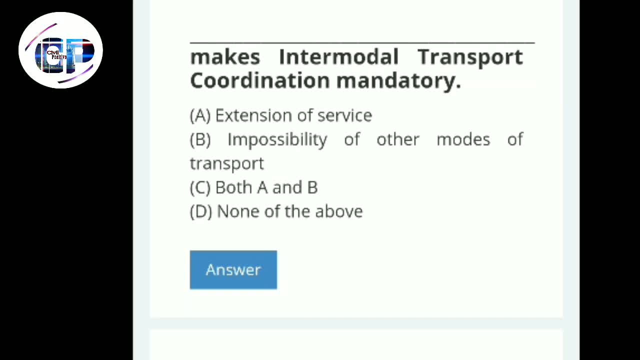 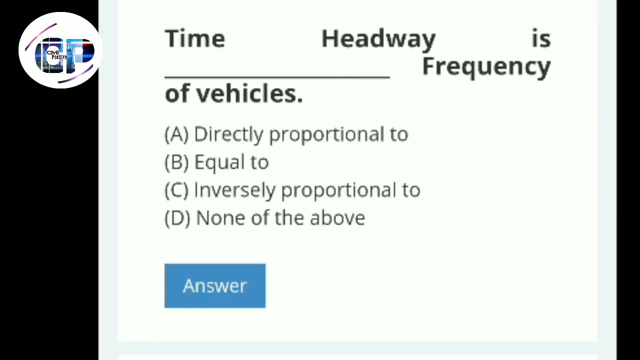 Impossibility of other modes of transport, both A and B. none of the above. Answer C: both A and B are right Time headway. is dash frequency of vehicles Directly proportional to, equal to inversely proportional to none of the above? 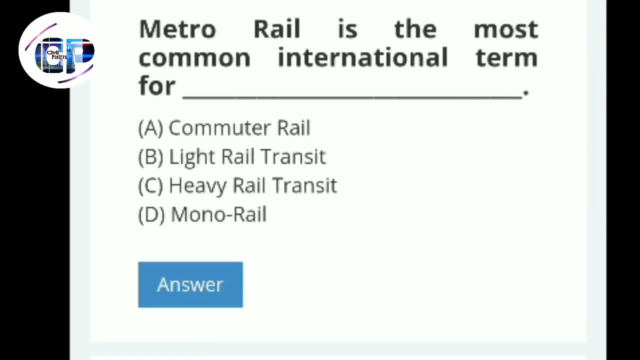 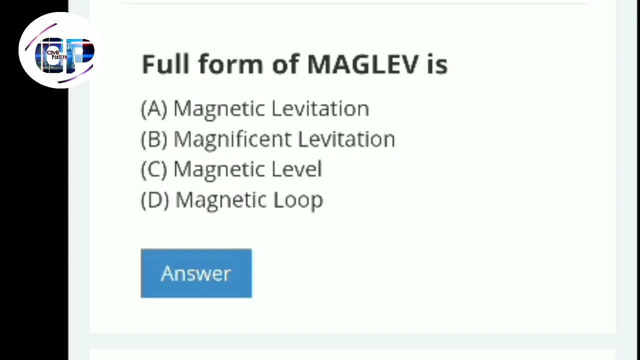 Answer C is right. inversely proportional to Metrodial is the most common international Term for dash Commuter rail. light rail transit, heavy rail transit, monorail. Answer C is right. heavy rail transit. Full form of MAGLEV is magnetic levitation, magnificent levitation, magnetic level, magnetic loop. 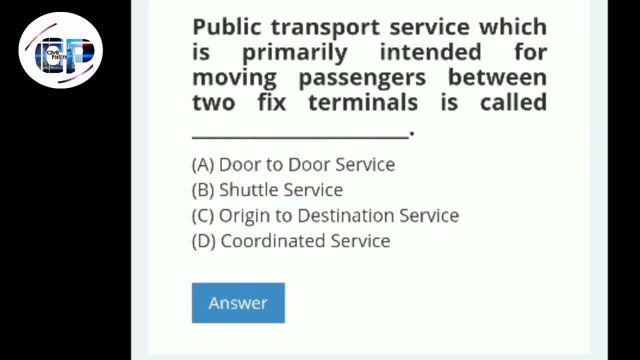 Answer A is right: magnetic levitation. Public transport service which is primarily intended for moving passengers between the two fixed terminals is called dash: Door to door service, shuttle service. origin to destination service, coordinated service. Answer B is right: shuttle service. 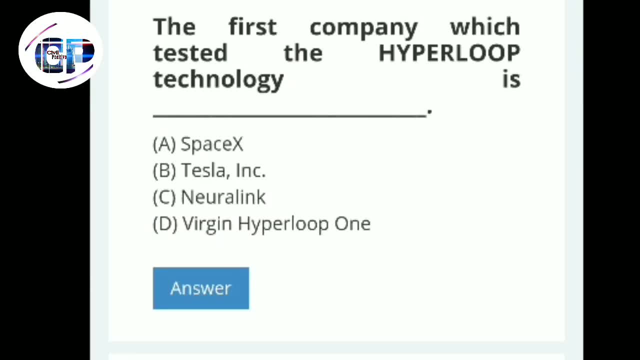 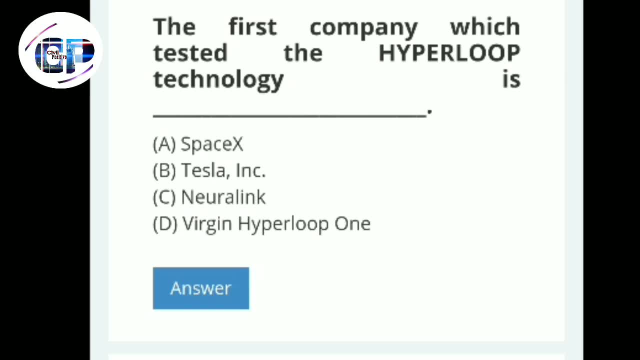 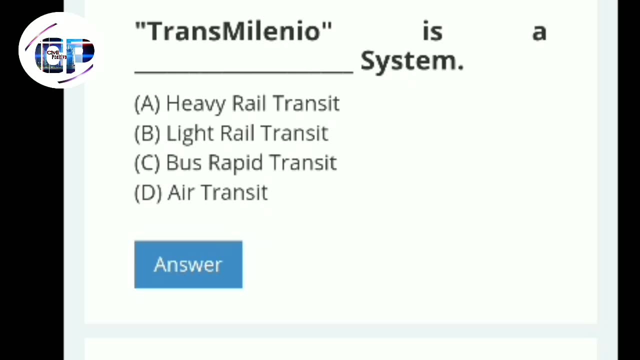 Space X- Tesla in New Relic Link: Virgin Hyperloop One. Answer D is right: Virgin Hyperloop One. Transmillino is a dash system: Heavy rail transit, light rail transit, bus rapid transit, air transit. Answer C is right: bus rapid transit. 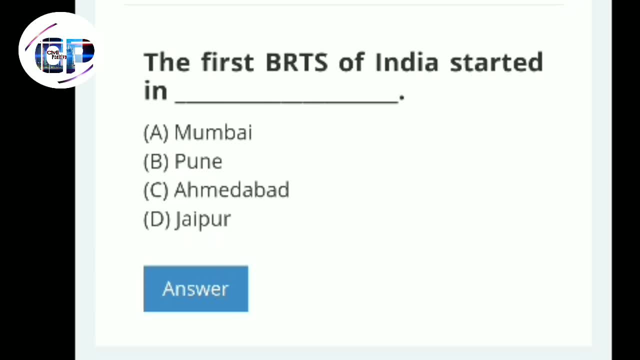 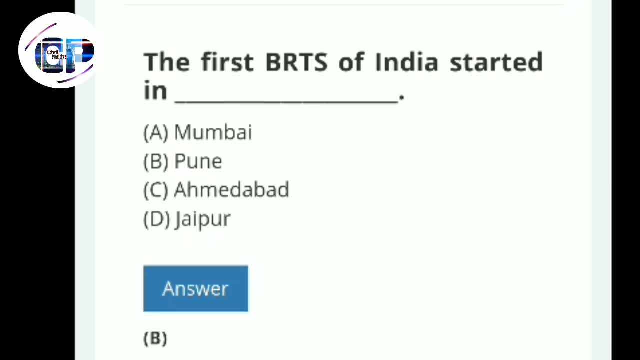 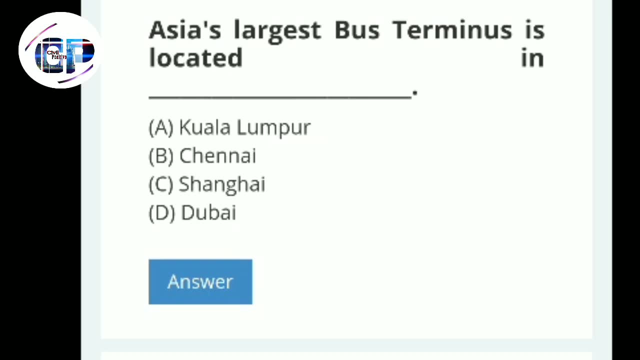 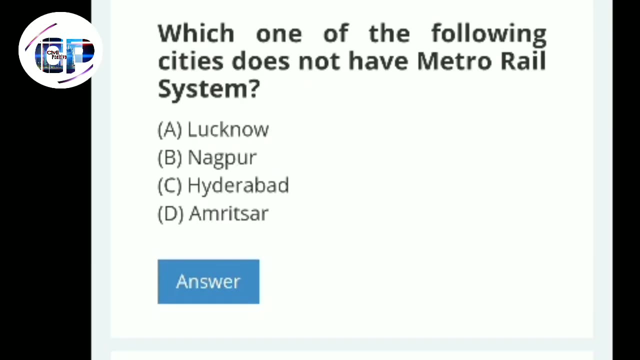 Answer B is right: Pune. Asia's largest bus terminal is located in D Kuala Lumpur, Chennai, Shanghai, Dubai. Answer B is right: Chennai. Which one of the following cities does not have metro rail system? A Lucknow, B. Nagpur, C. Hyderabad, D- Amritsar. 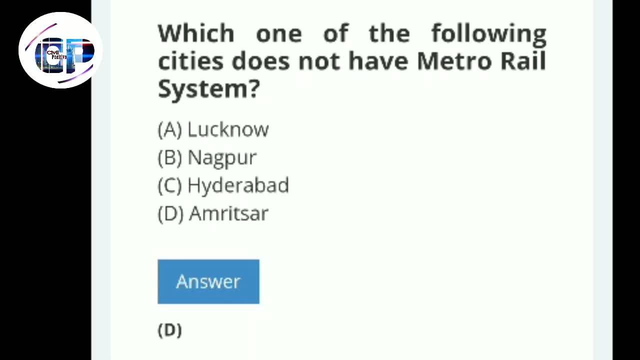 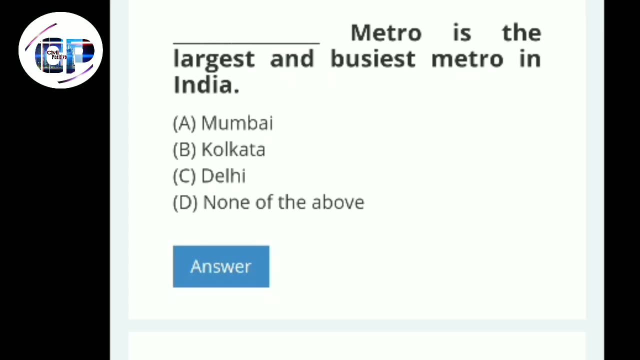 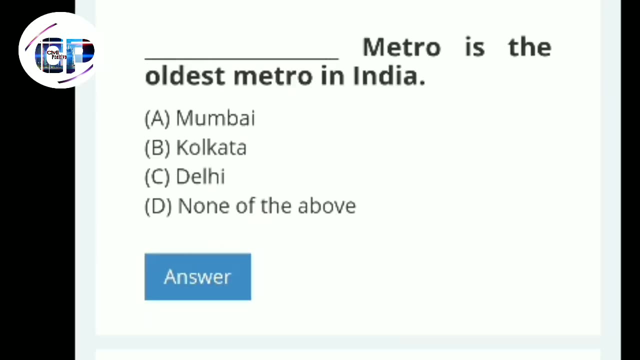 Answer D is right. Amritsar D Metro is the largest and busiest metro in India. A- Mumbai, B- Kolkata, C. Delhi D. None of the above. Answer C is right. Delhi D Metro is the oldest metro in India. Which one of the following cities does not have metro rail system: A- Mumbai, B- Kolkata. C- Delhi. D- Delhi. A- Kolkata is right answer: B- The Indian Government has approved the version. Hyperloop owns plans to develop a high-speed line between: 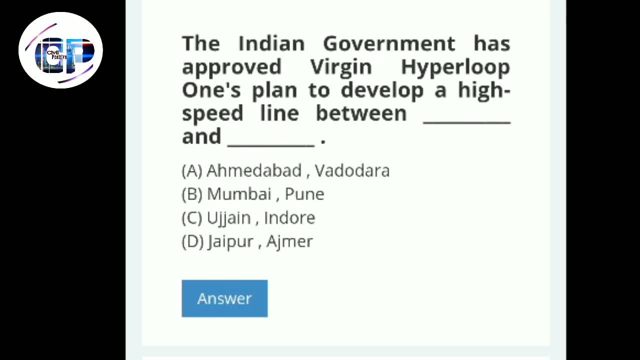 D S and D S. Where was the first high-speed plan? A Ahmedabad, B Varodara, C Mumbai, Pune. A Ujjain, B Indore, C Jaipur, A Ajmer. 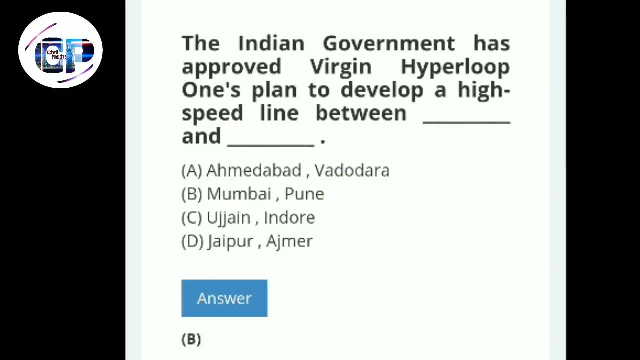 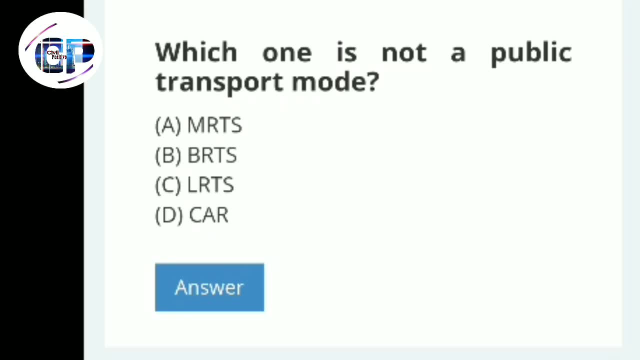 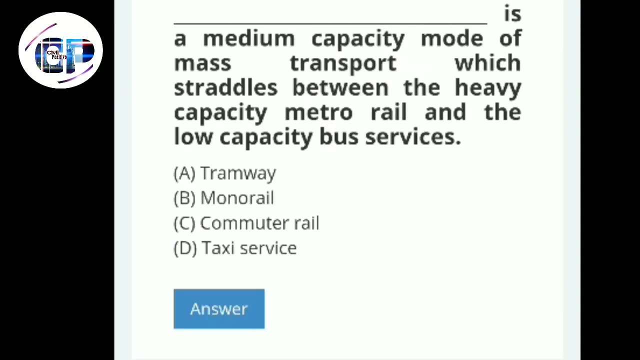 Answer B is right: Mumbai, Pune. Which one is the not a public transport mode- mrts, brts, lrts, car? answer d is right: car. this is a medium capacity mode of mass transport which strategies between the heavy capacity- metro, rail- and the low capacity? 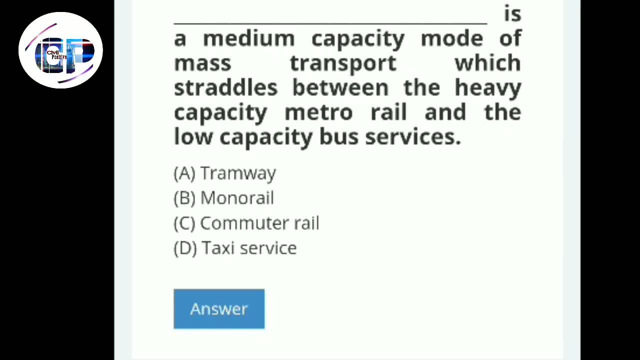 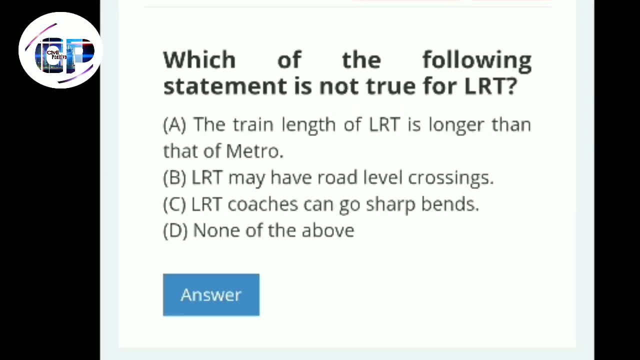 bus service, tramway, monorail, commuter, rail, texas service? answer a is tramway. which of the following statement is not true for lrt? first option: the train length of lrt is longer than date of metro. lrt may have road level crossing. lrt coaches can go. 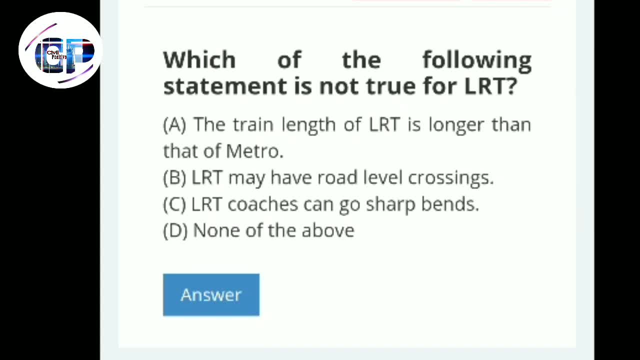 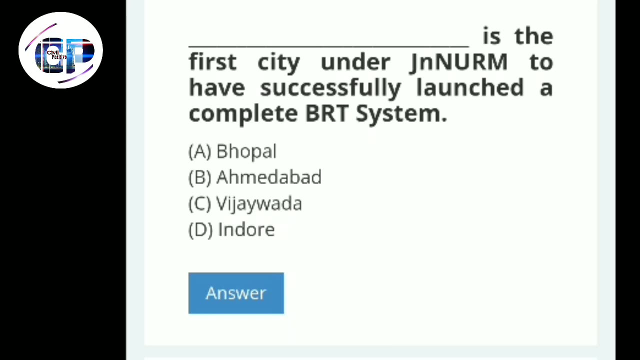 bends. none of the above answer is right. the train length of lrt is longer than data. metro rail is the first city under the gene neurone to the have successful launch a complete brt system: popal, amdavad, vijayavada, indoor. answer b is right: amdavad. 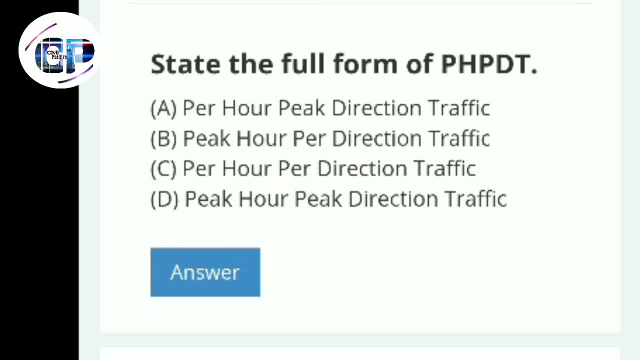 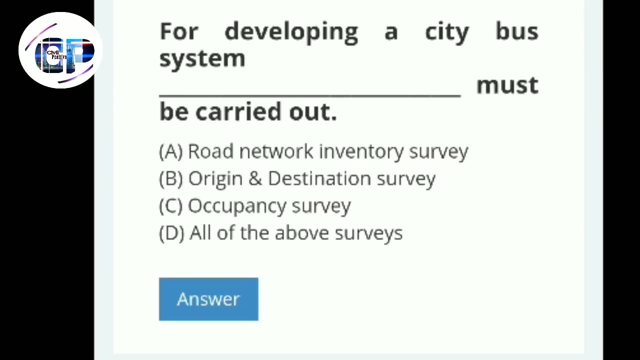 state the full form of phpdt: per hour. peak direction traffic. peak or per direction traffic. peak or per direction traffic. peak or peak direction traffic? answer d is right. peak or peak direction traffic for developing a city bus system? this must be carried out: road network inventory survey, origin and destination survey, occupation survey, all of the 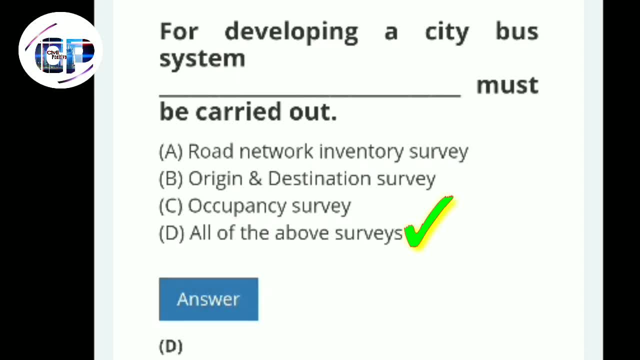 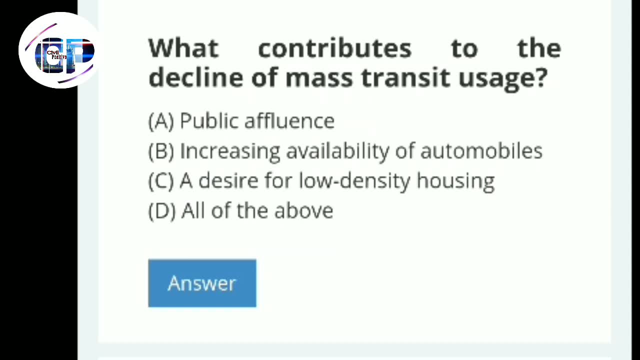 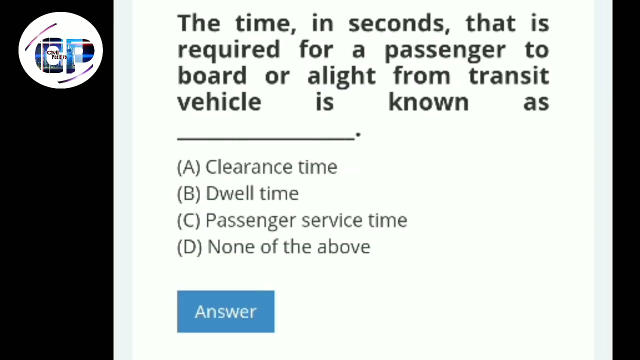 above survey? answer d is right. all of the above survey. what contributes to the decline of mass transit uses? public influence, increase the availability of automobiles, a desire for the low density housing? all of the above? answer d is right, all of them. the time in second that is required for a passenger to